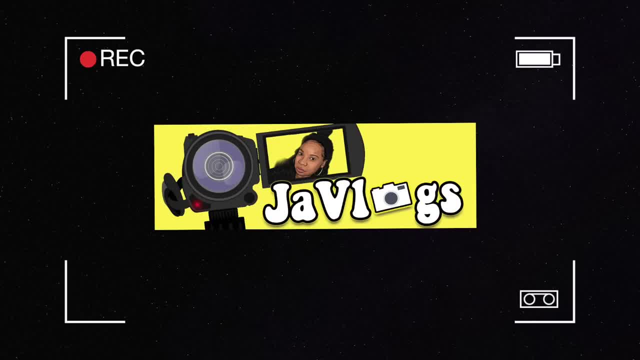 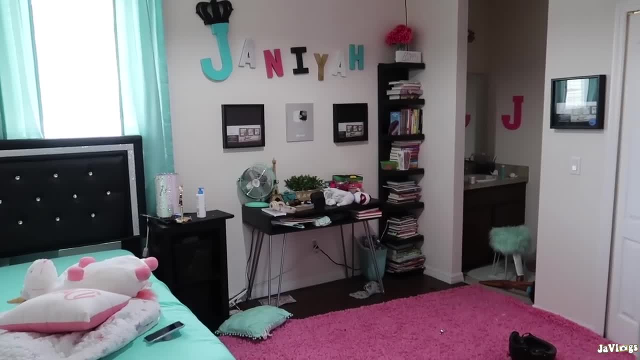 What's up y'all? So I told you that I was going to be rearranging Naya's room, So that's what I'm about to do. So this is what it looks like before. Hi, So this is coming. 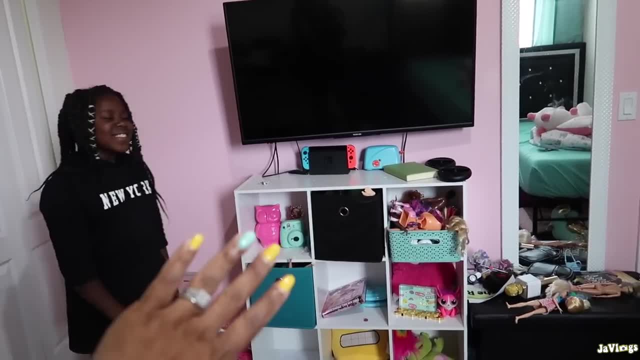 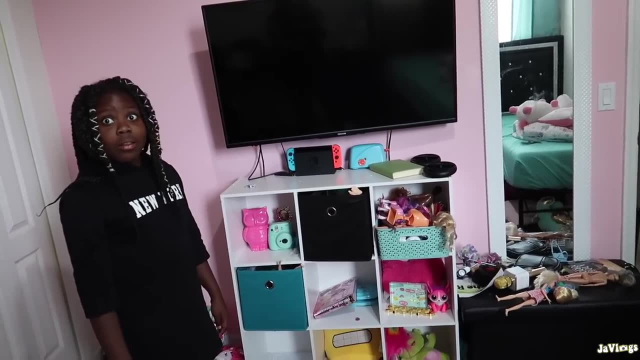 out of here Out And we're going to put her Barbie house. I hope your Barbie house ain't too tall, is it That ain't going to be tall as a TV? No, it shouldn't be Uh-huh, Do you? 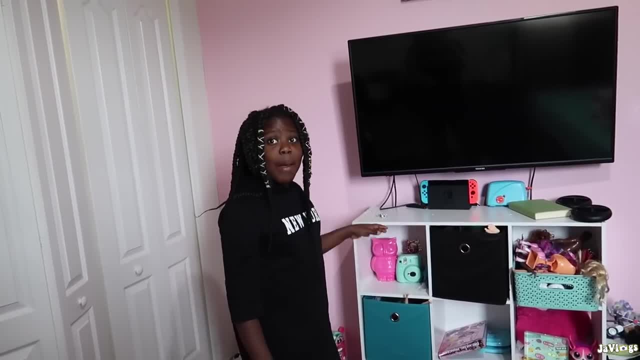 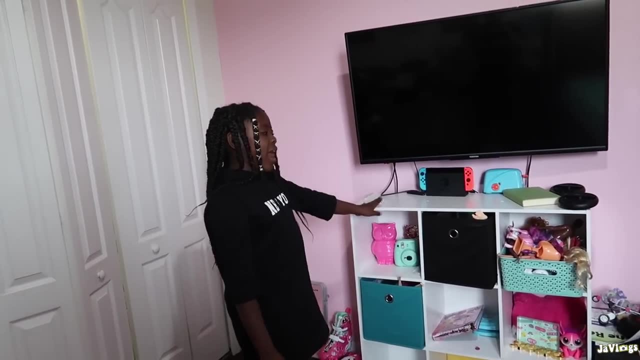 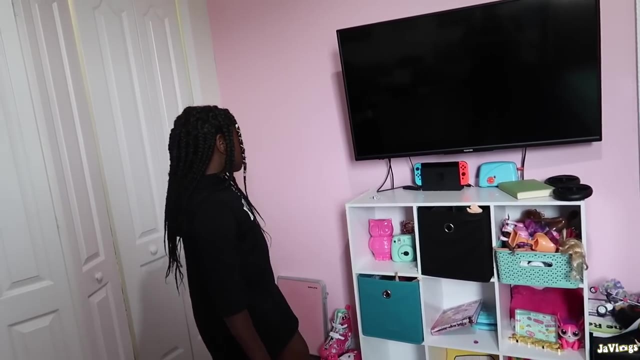 think so Yeah, it's taller than this. I think that part like the upstairs, Oh, we're going to have to measure, I ain't even think about that. So you're going to get your dad It's taller. Oh man, I thought we were smooth. I was getting geek like, oh okay, we can. 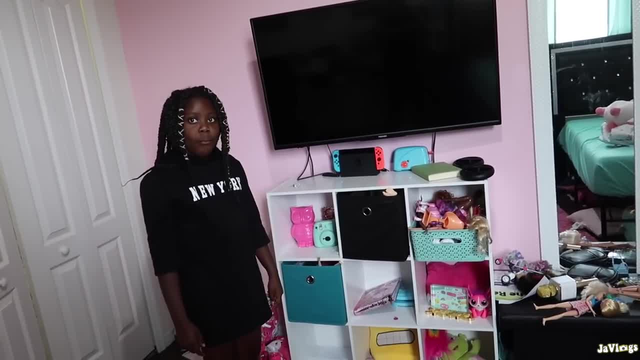 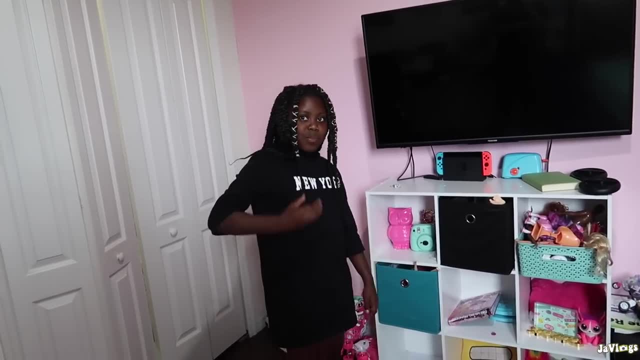 just move this out of the way, because this is the whole reason why I'm rearranging her room to fit her Barbie house. She loves Barbies or any kind of like dolls, But the Barbie house is going to be taller than this, So we're going to have to measure. I ain't. 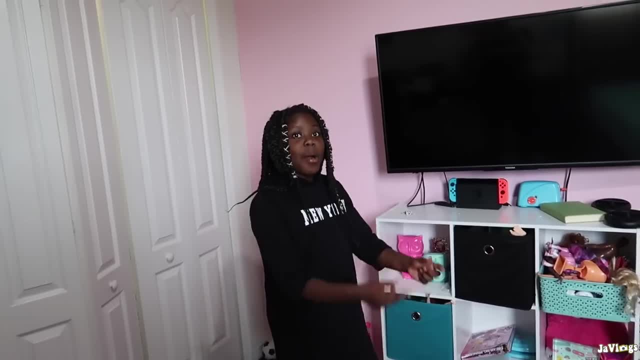 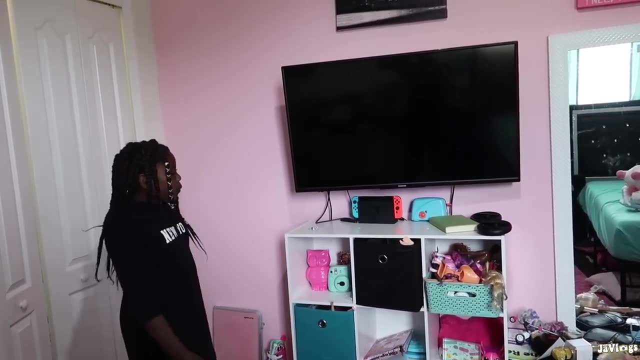 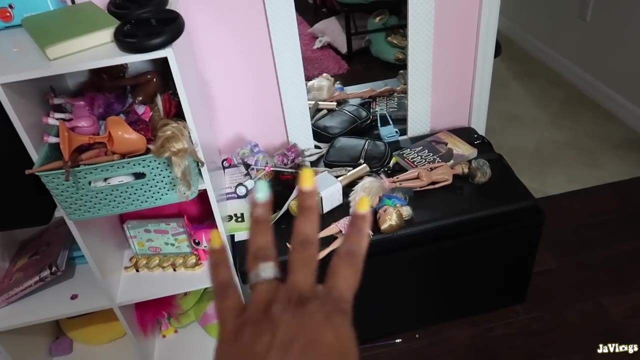 not baby dolls Like Barbie dolls, Yeah, but they all don't. Yeah, they get the point. They get the point. Also, as y'all know, right now her Barbie house is outside on the patio, So I'm tired of Barbies everywhere. She got Barbies here. She got them all over the place. 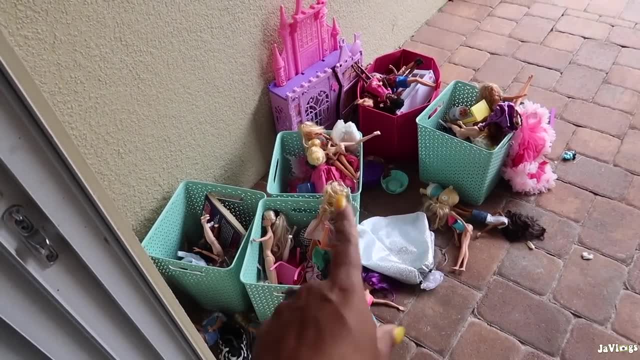 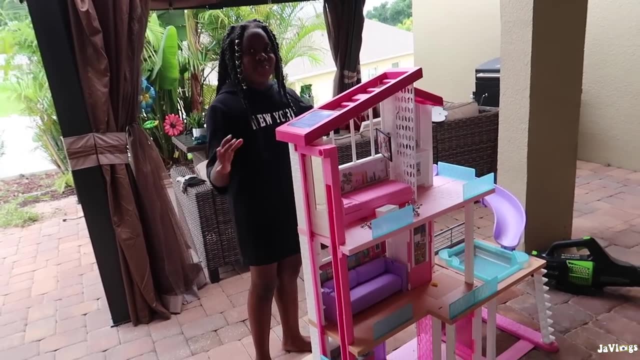 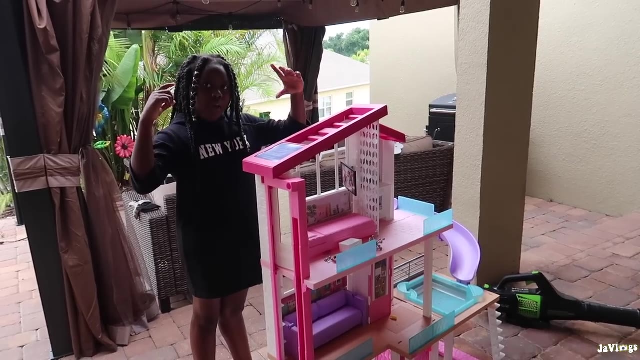 here. This is currently where her Barbie's been stationed for a couple months now. I think that's too tall. Yeah, that's way too tall. Wow, Yeah, that part Dang. I thought we had something We're going to have to figure. Move out the TV, Like you know, how you like. 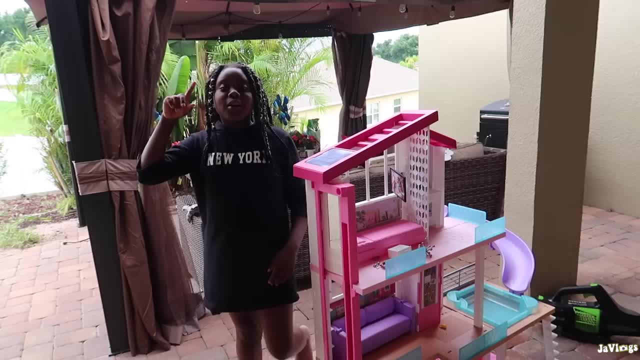 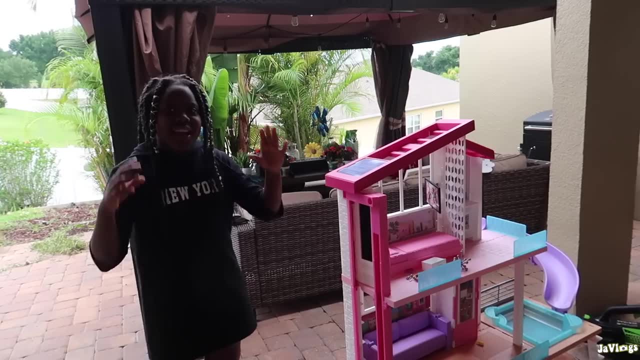 What We can't. The TV is on the wall. We can't do nothing with the TV. I know I'm talking about like move it out And put it like behind it, Behind it. Okay, that may be a good idea. 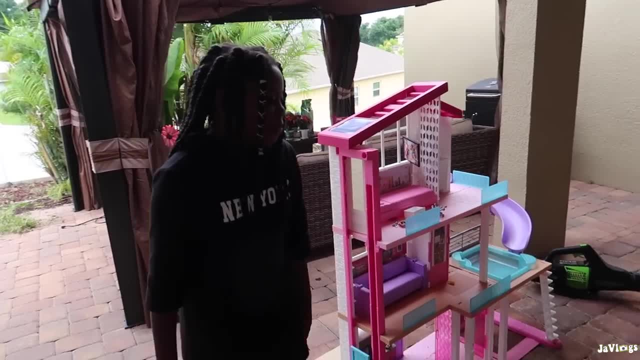 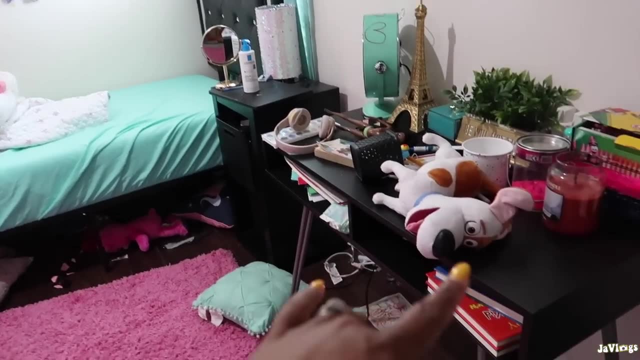 And then behind it just fucking up there. We're going to have to figure out something. We're going to have to figure out something. So we're going to change her bed around. Probably, going along this way, We're going to move this out. All the wall decor is staying. Well, I may move this, This. 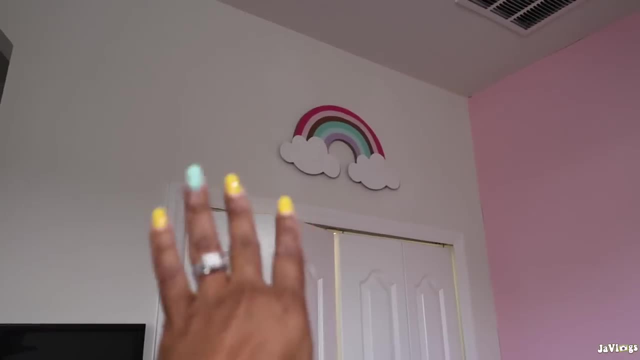 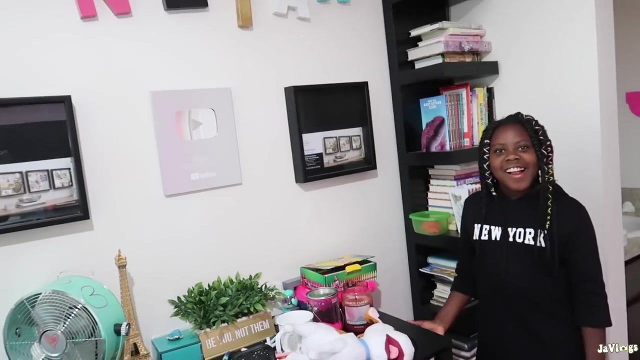 here is definitely staying. This stuff is going to stay That. We've been here what six, seven months and I still ain't put nothing in these boxes. Are we going to use it or not? Right, So we're going to do that today. 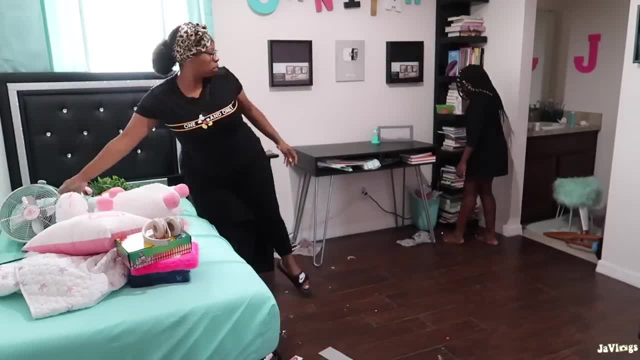 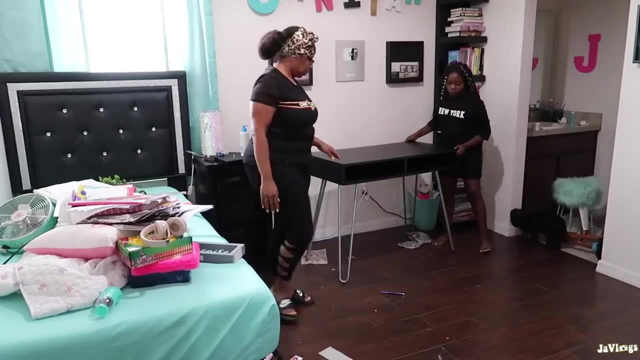 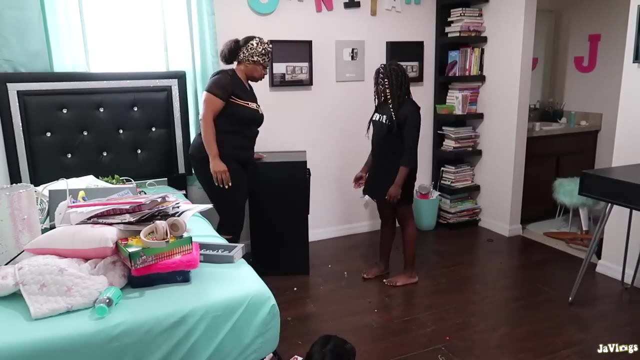 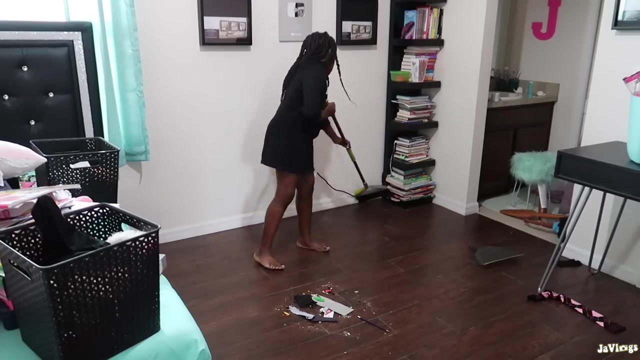 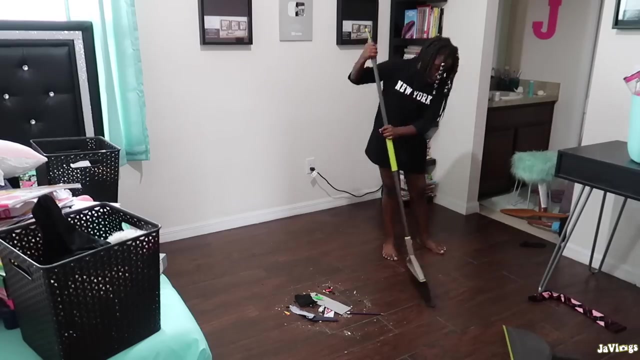 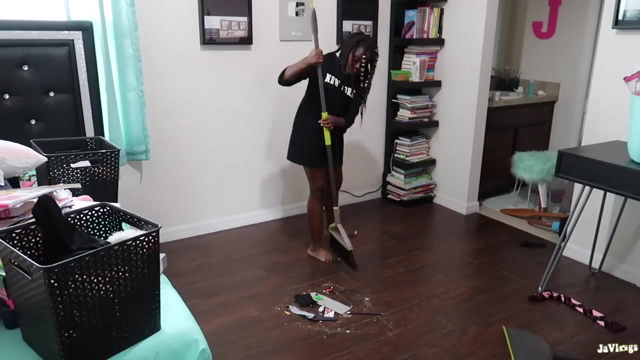 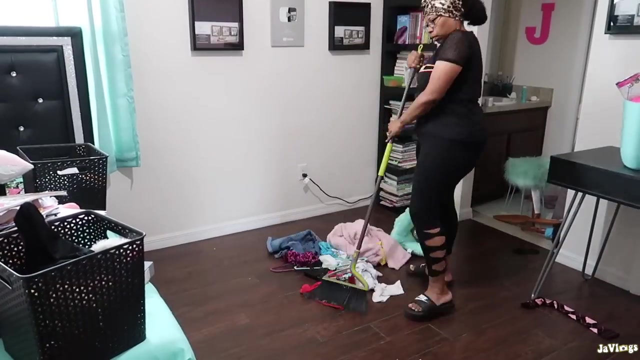 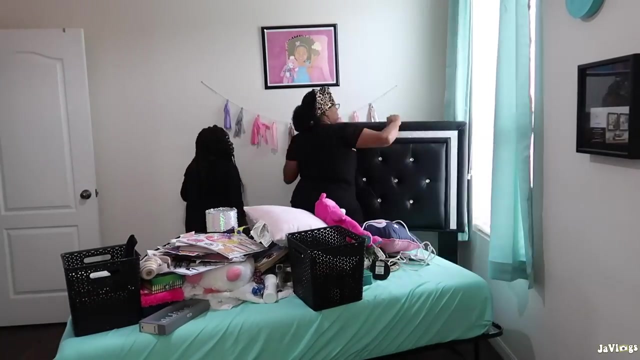 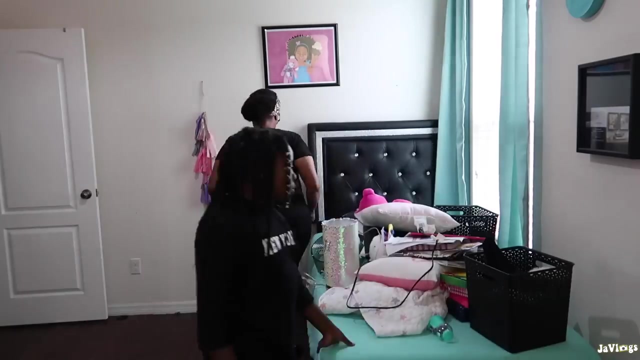 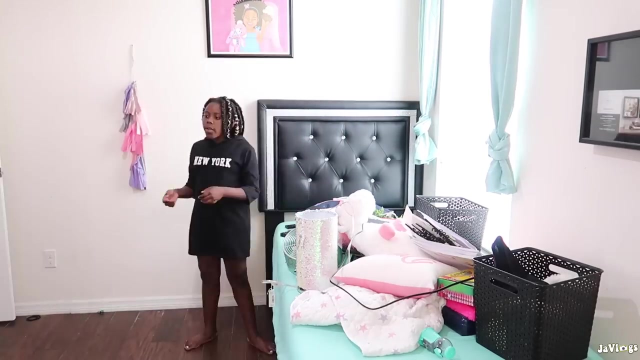 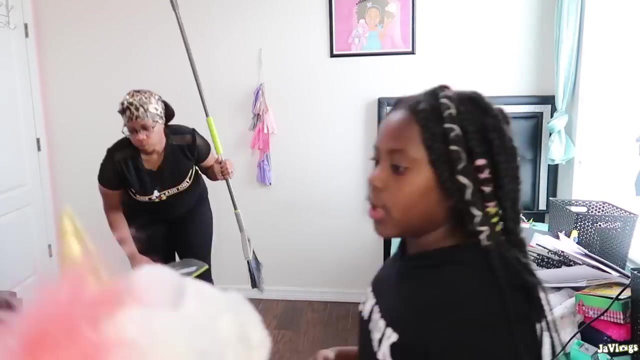 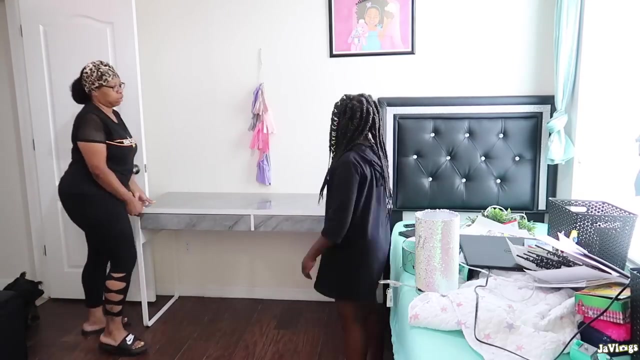 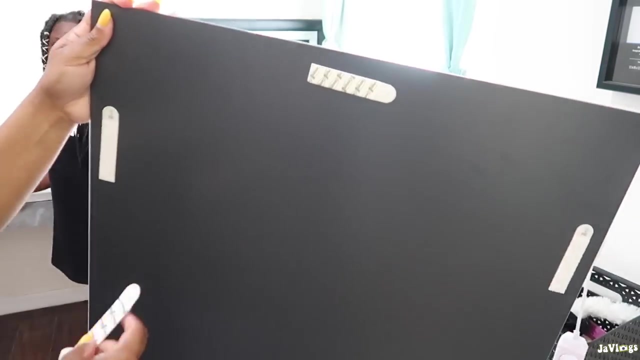 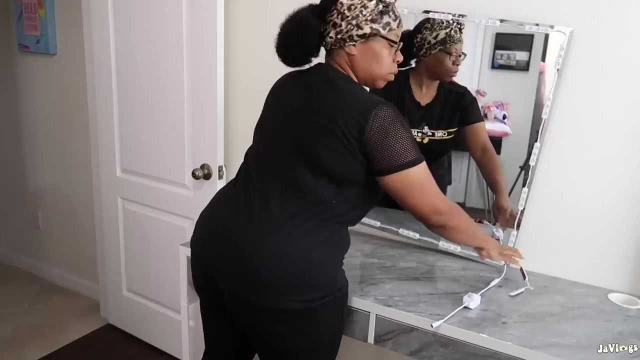 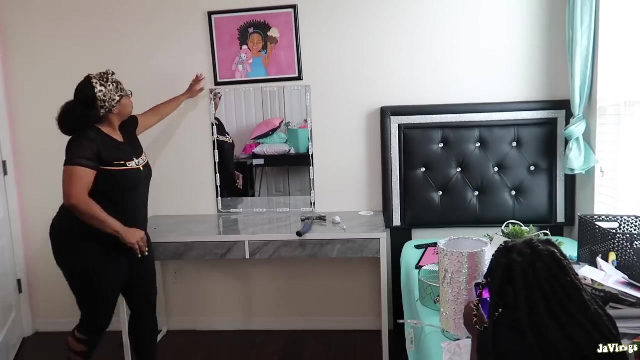 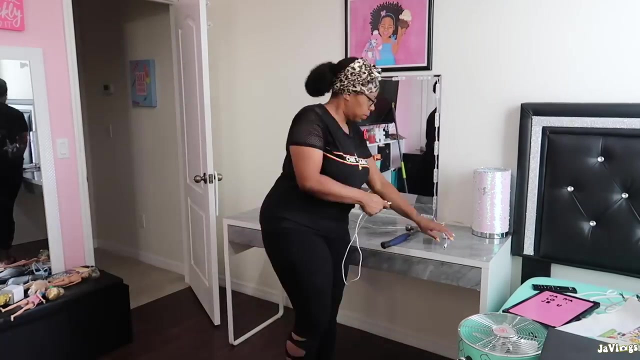 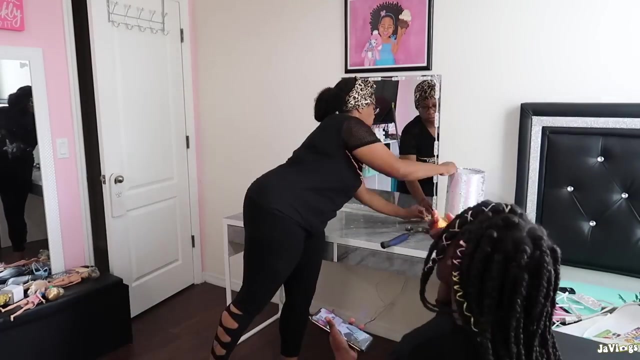 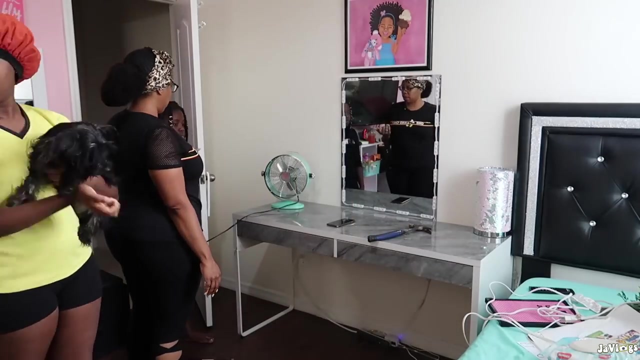 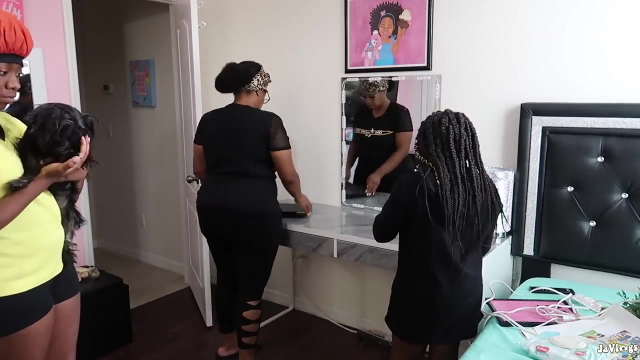 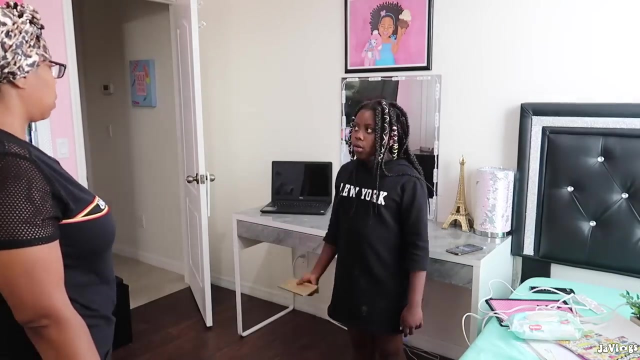 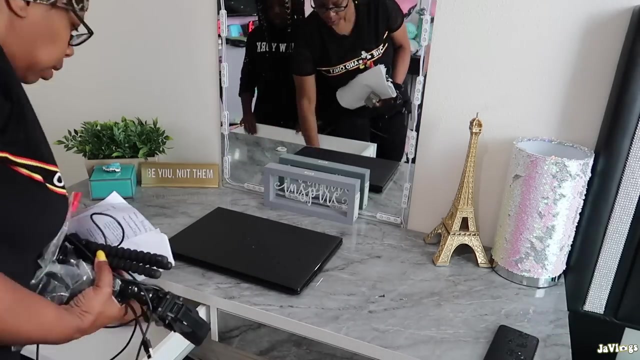 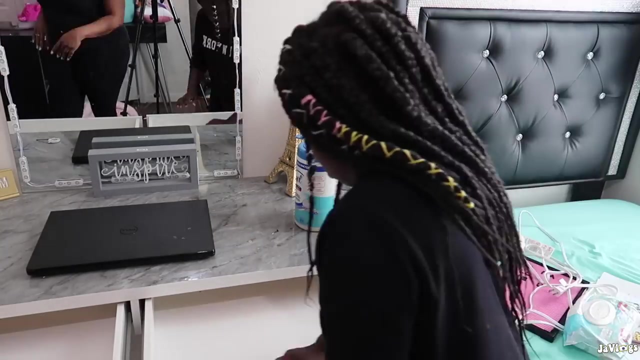 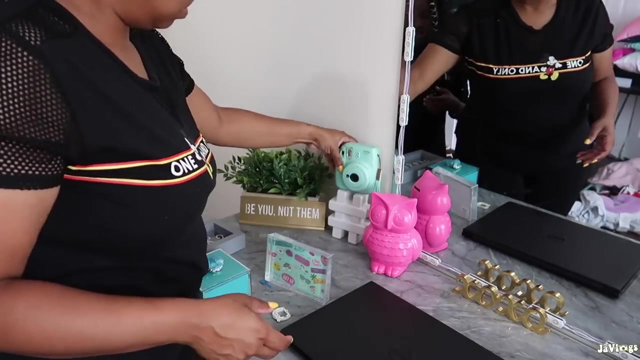 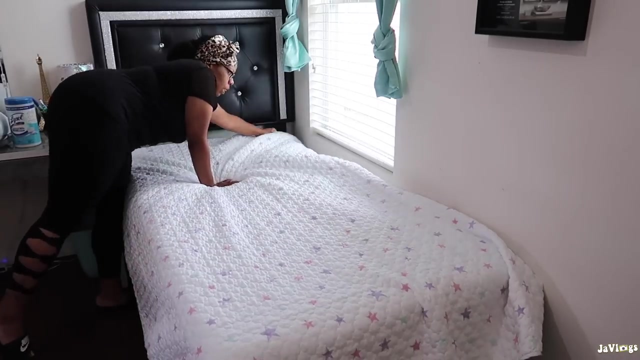 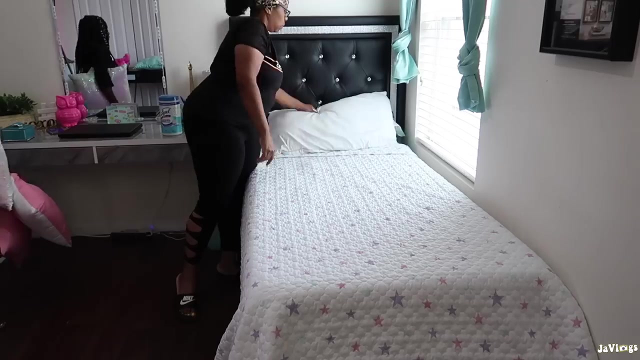 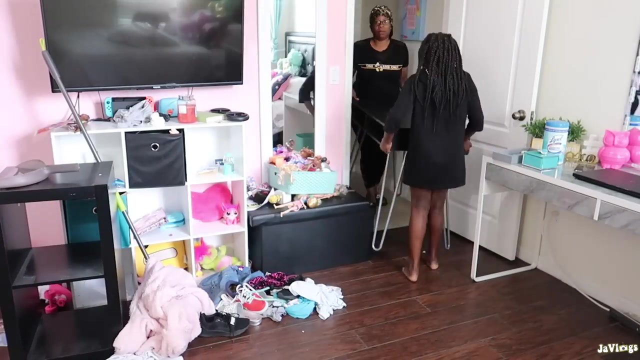 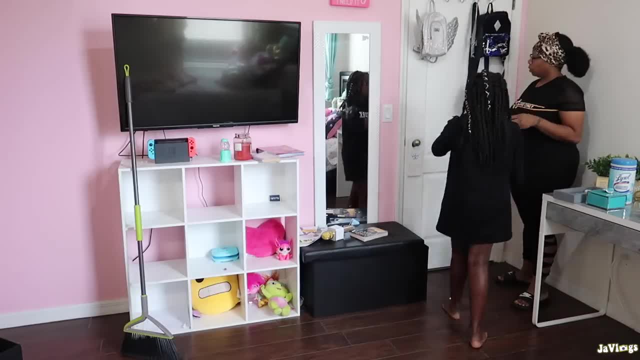 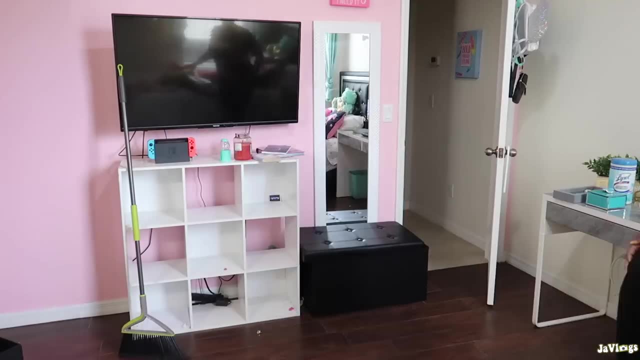 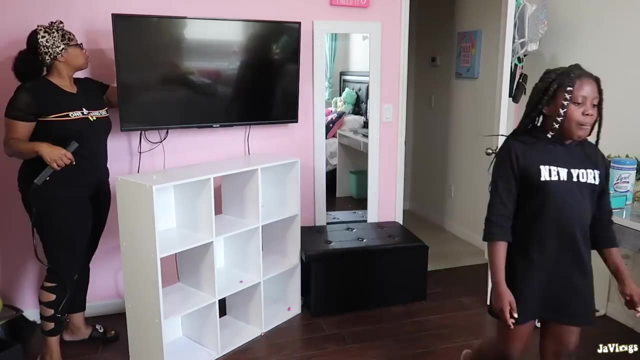 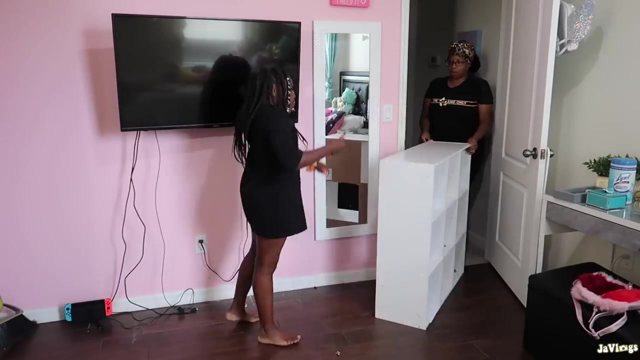 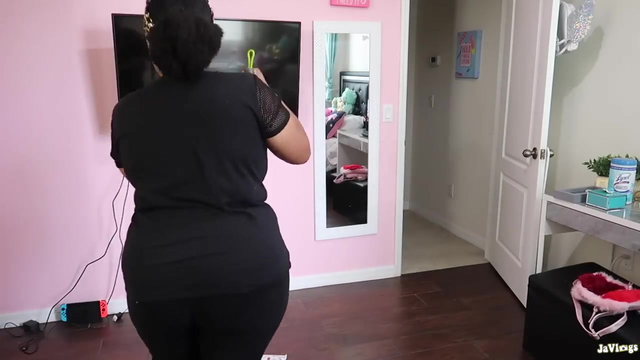 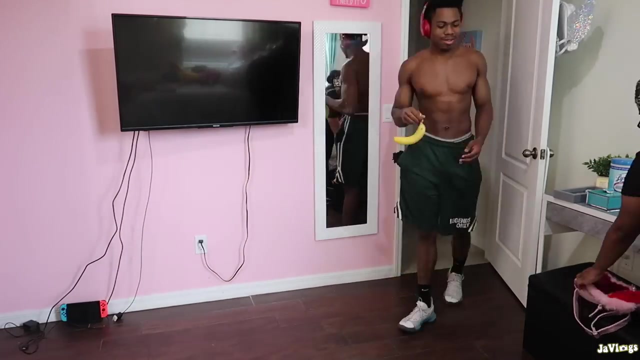 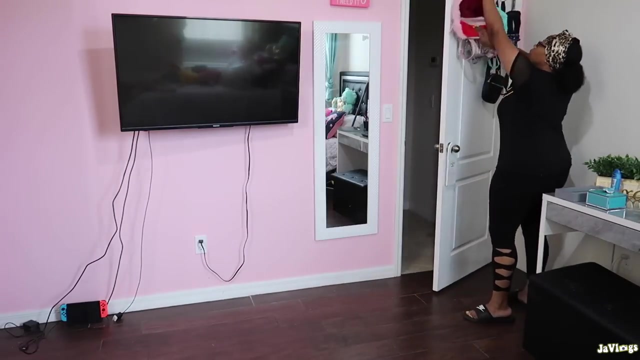 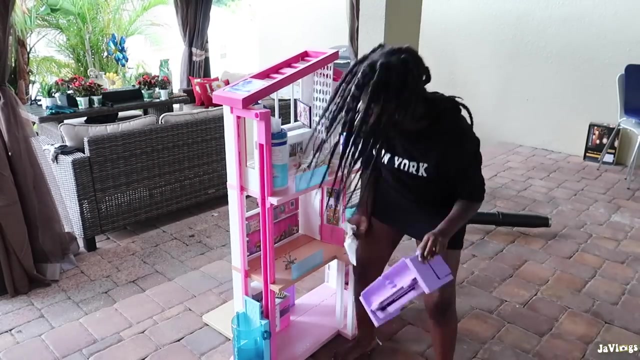 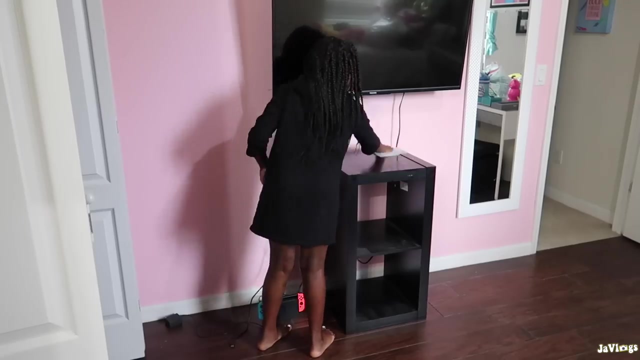 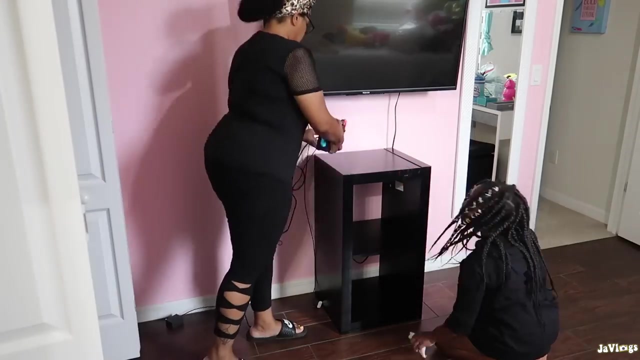 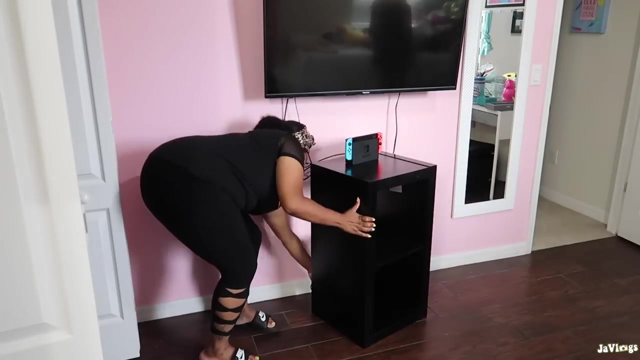 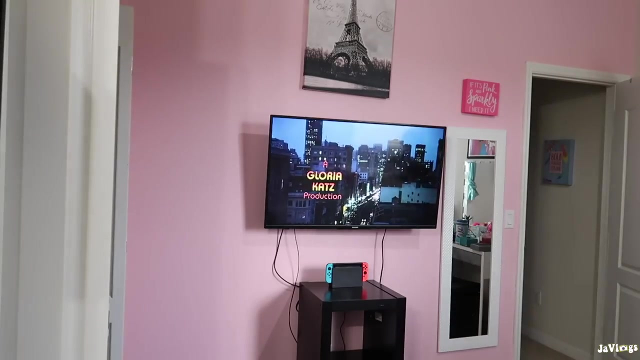 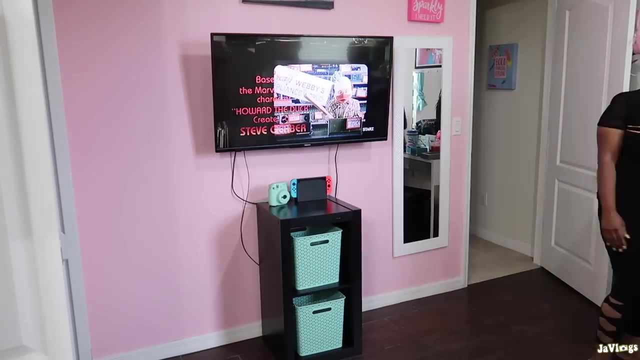 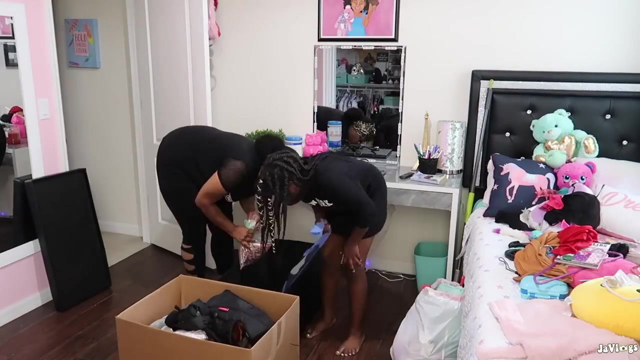 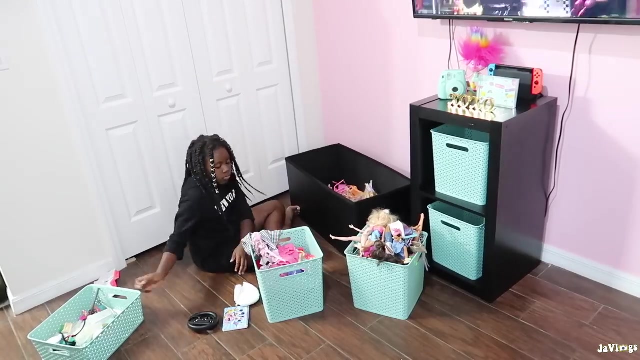 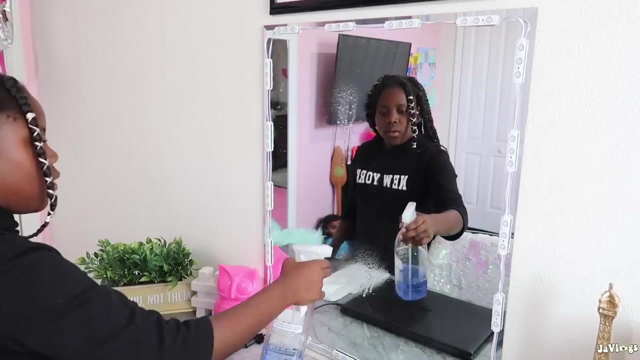 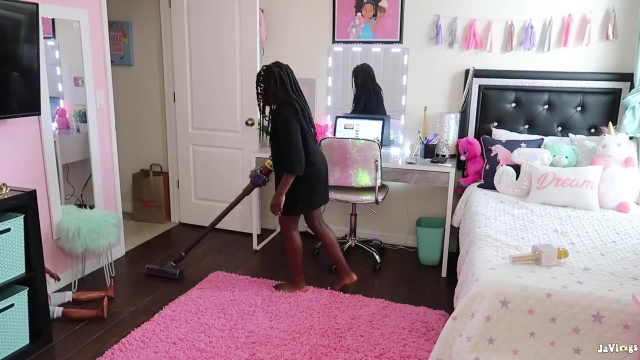 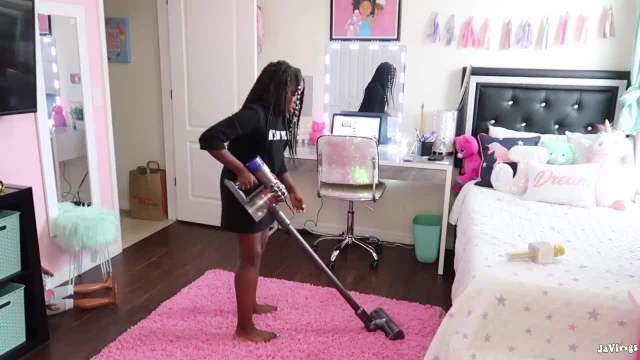 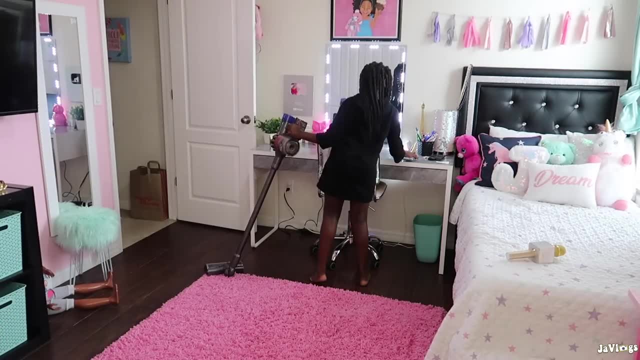 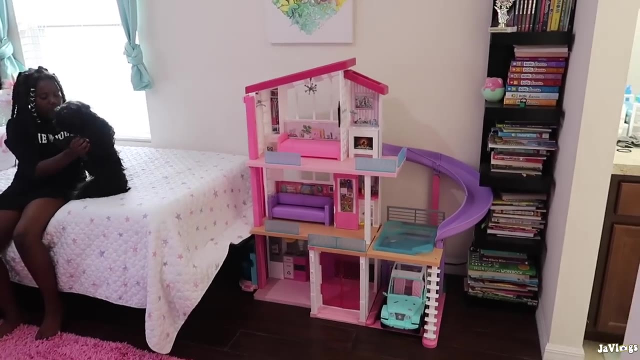 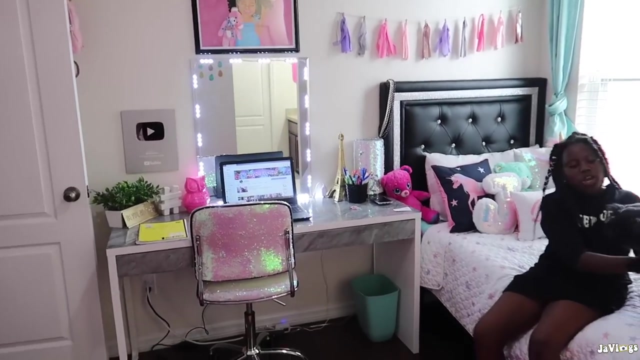 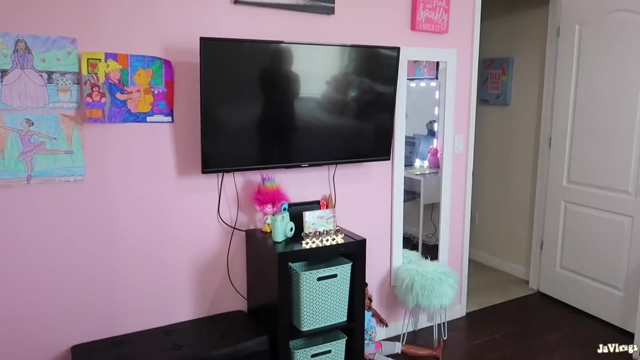 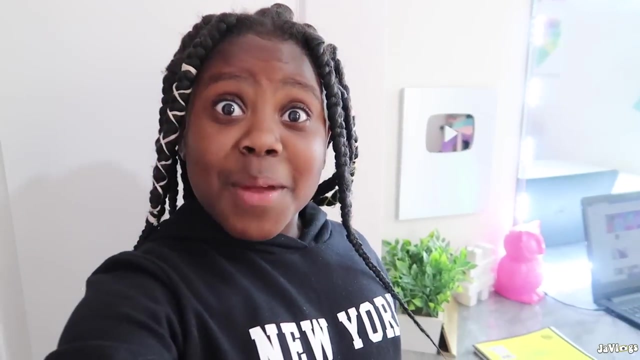 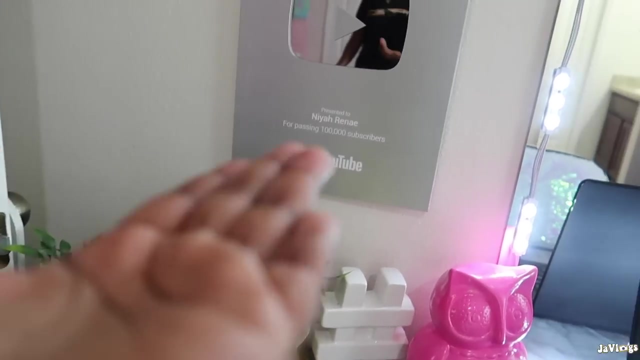 So we're going to do that today. So we're all done with my room. So now I'm going to give you guys a tour. So here's my desk right here. I got a little bit of decor. My plaque right here. 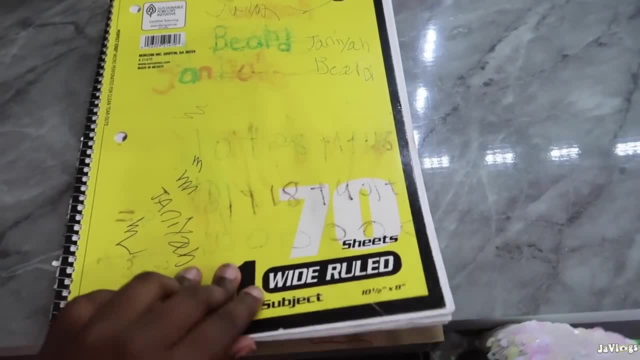 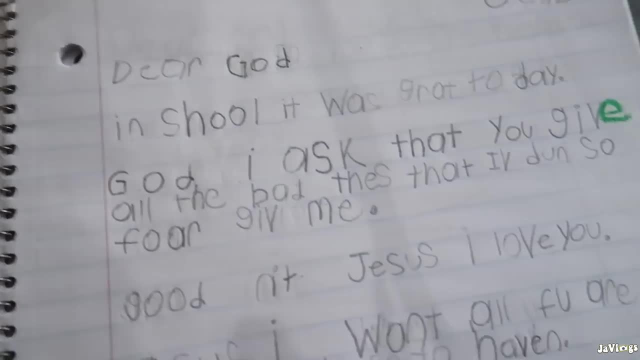 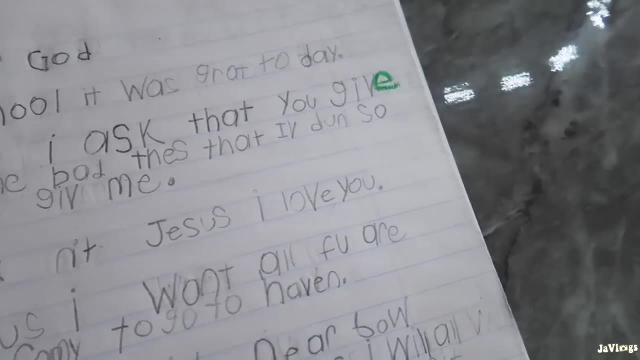 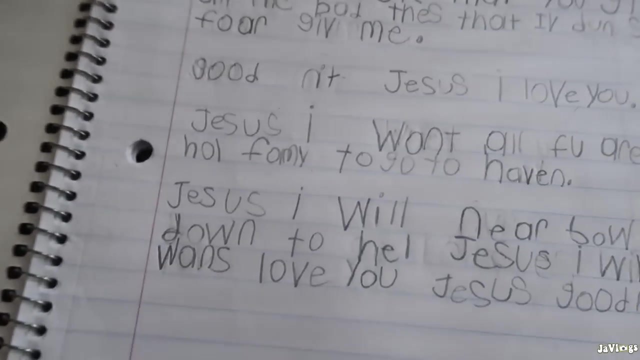 I found this notebook that I had for a really, really long time. I want to show you guys what's in it. Yeah, in kindergarten It says Dear God, in school it was great. today, God, I ask that you give all the bad times that I've done. So forgive me, Good Jesus, I love you. 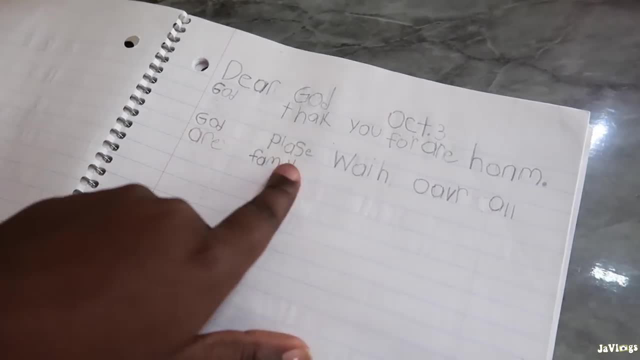 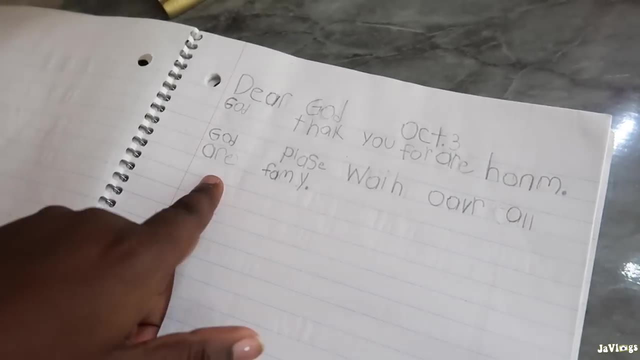 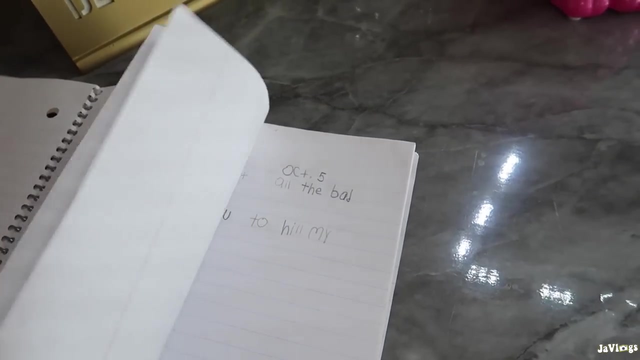 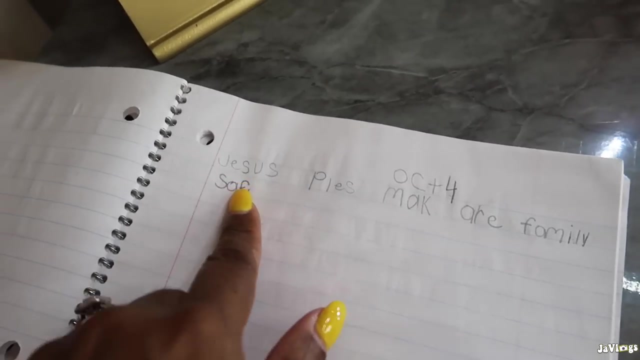 Dear God, thank you for our home. God, please watch over all our family, Mind you y'all. this was kindergarten, It's spelling, It's cringy. It says: Jesus, please make our family safe. Where did you get that, though? 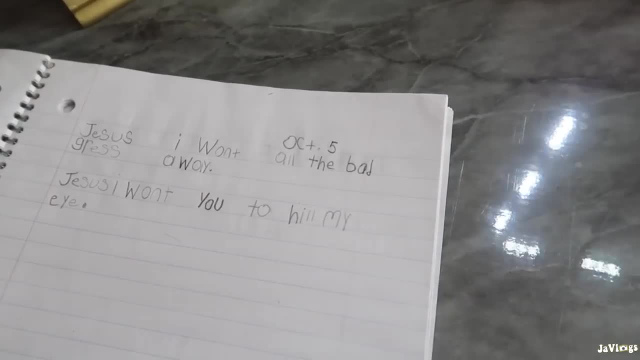 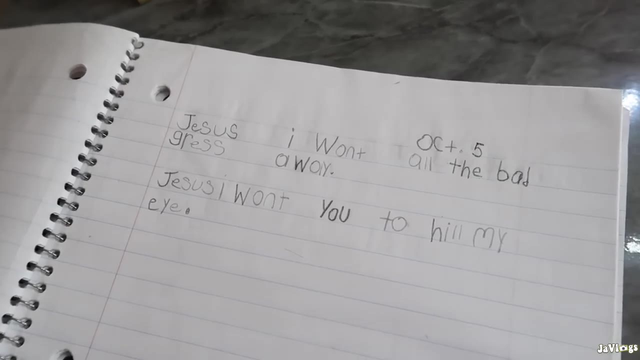 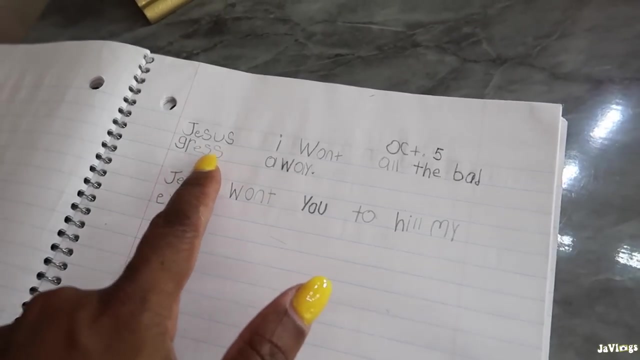 My plaque. My plaque: Jesus, I want all the bad Grease away. Jesus, I want all the bad grease away. I think she was talking about grades, But I got good, though I don't know why she said that She always got good grades. 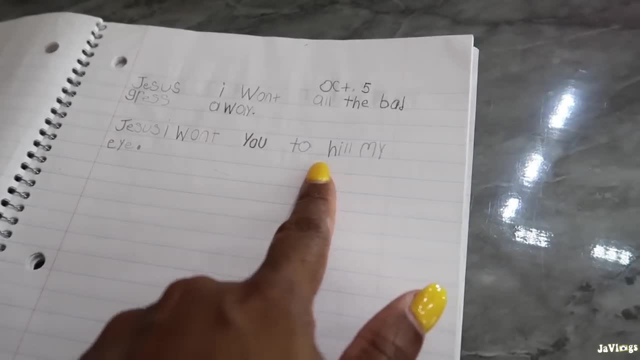 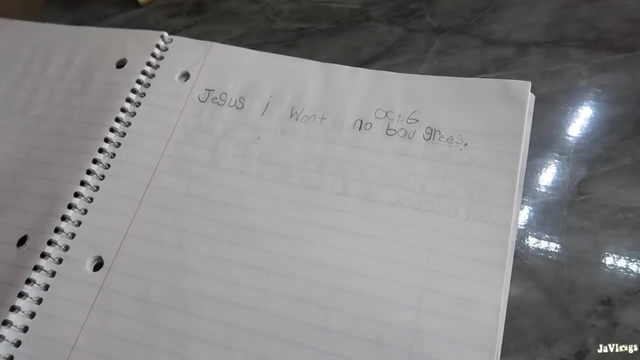 I don't know. I don't know, Jesus, I want you to heal my eye. We don't know what's wrong with my eye, So something must have been wrong with her eye on October 5th. Jesus, I want no bad grades. 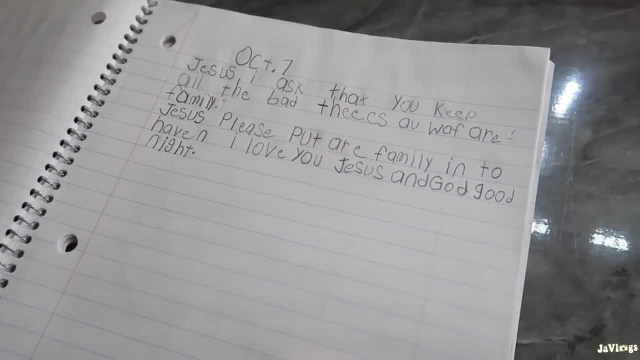 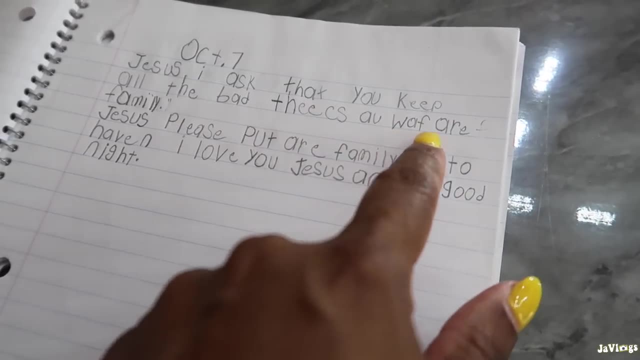 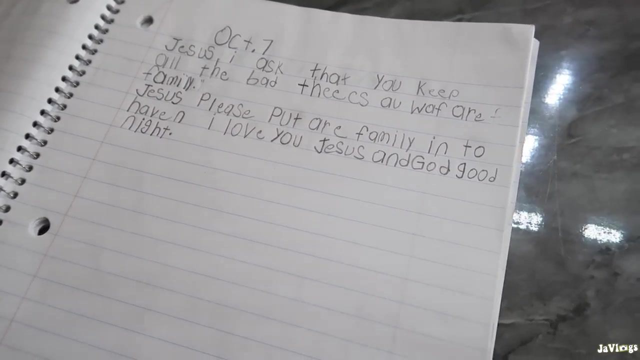 Jesus, I ask that you keep all the bad- What's that? Feet, Feet, Feet, Wait huh- All the bad Things away from my family. I don't know. Okay, I guess. so, Jesus, please put our family in heaven. I love you. 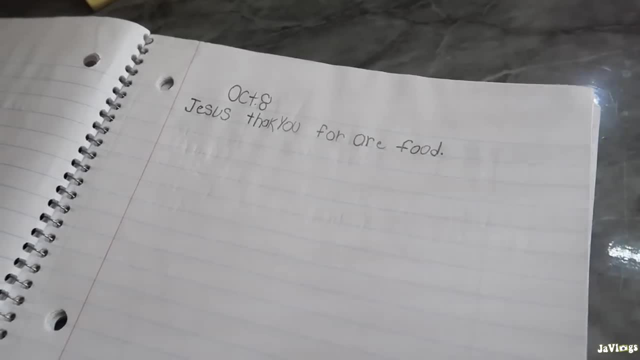 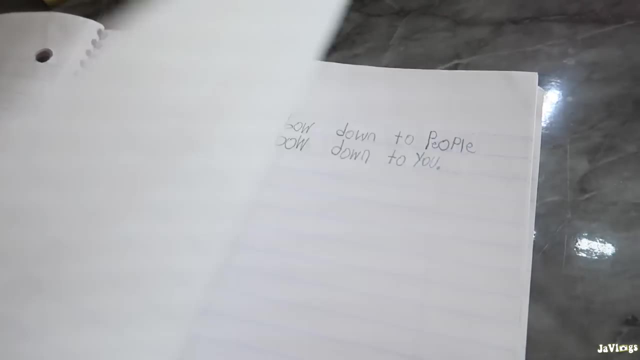 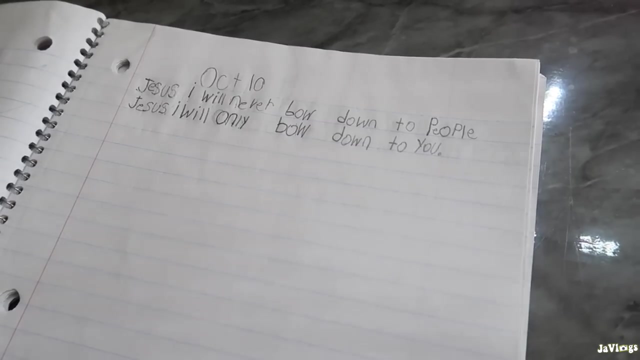 Jesus and God. good night, Jesus. thank you for our food. Lord, I ask that you forgive me my sins. Jesus, I will never bow down to people, Jesus, I will only bow down to you. We had fun at the dam and the park too. 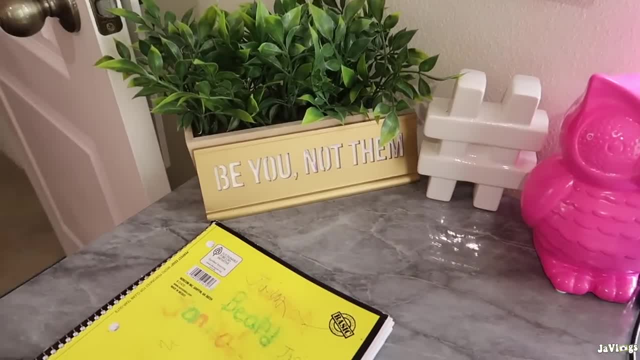 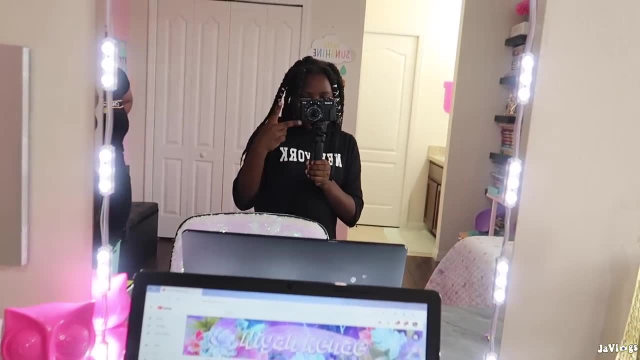 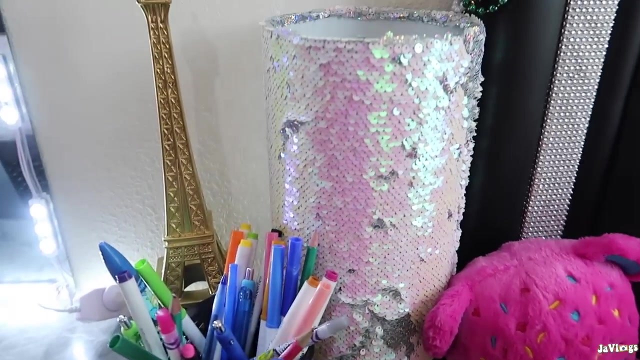 My life is fun too, So over here, yeah, I'm going to give you a closer look at the decor. And then we have my laptop right here, And then this mirror, And then this picture here I got from Etsy. And then over here we have this little lamp and it's sequins. 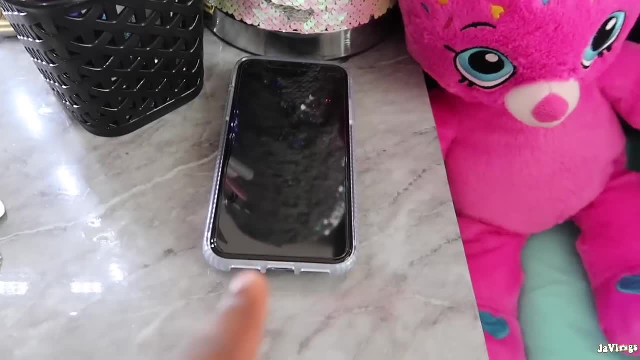 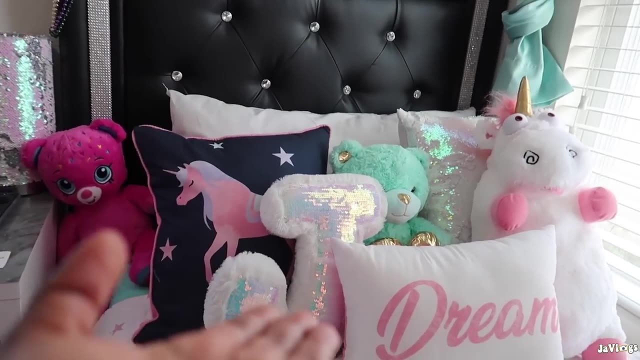 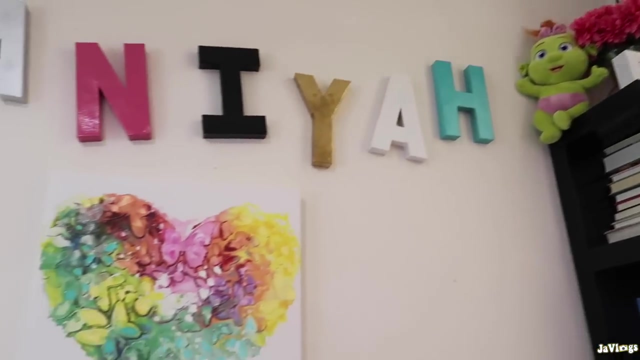 I have all my pins and markers and stuff. I have my phone right there, This little Paris decor, My bed. right there, I have a lot of stuffed animals. I have my pillows on here- Nothing new. And then, right here, I have my name spelled out: Janiyah. 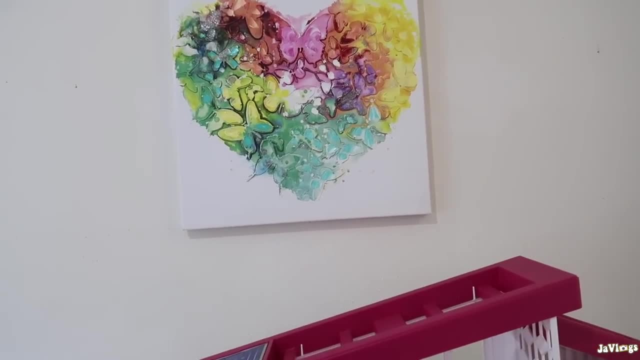 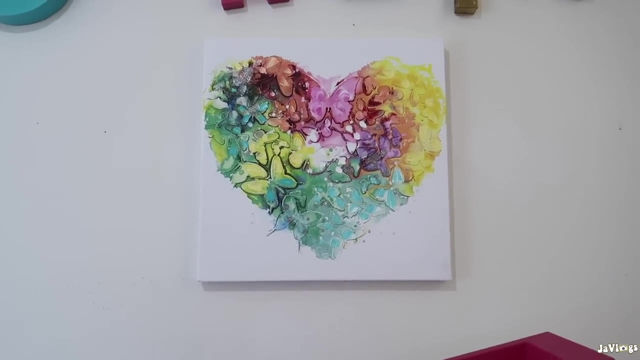 And then I have this little picture that came from Hobby Lobby. Hobby Lobby, Y'all originally put this outside, But I thought it was the perfect colors for her room And plus I took down those shadow boxes because we just didn't have nothing really to. 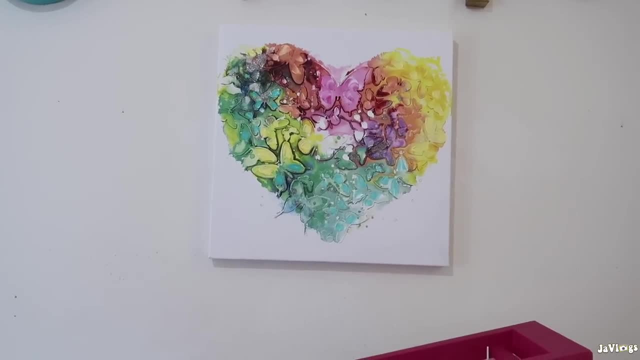 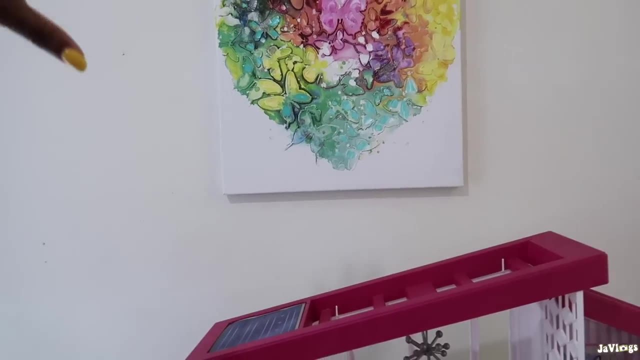 I just didn't feel like trying to find something to put in the doggone things, So I took those down. I took her YouTube plaque down, Put it over there, as y'all seen, But then I put that there because the colors is just perfect. 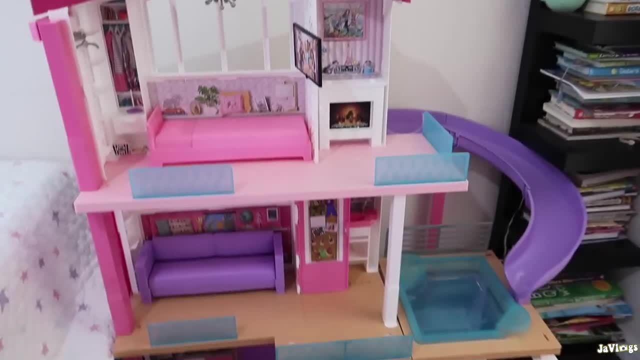 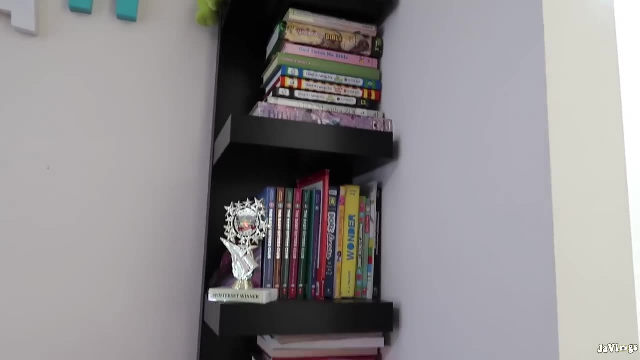 Yeah, It's really cute. I have my Barbie dream house in here- Finally got it to fit- instead of outside all the time. And then I have my bookshelf. Nothing new, Just a lot of books. Okay, So we have this Hello Sunshine thing from Hobby Lobby. 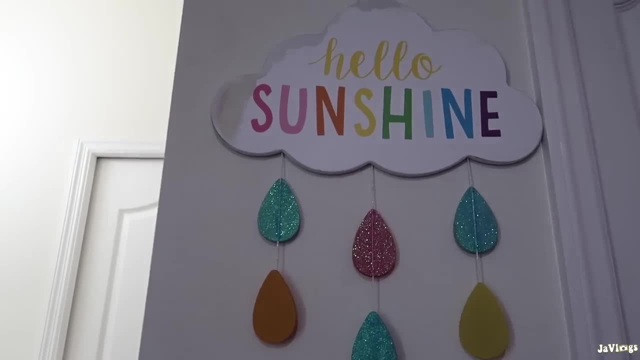 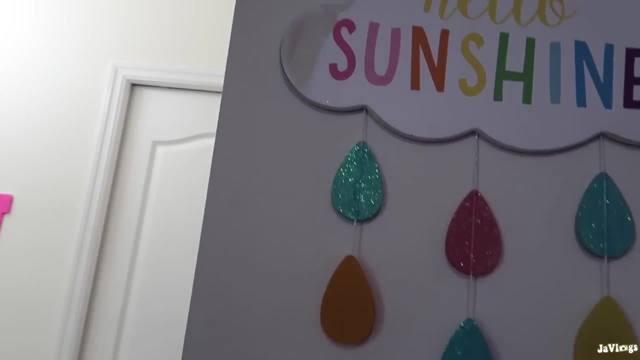 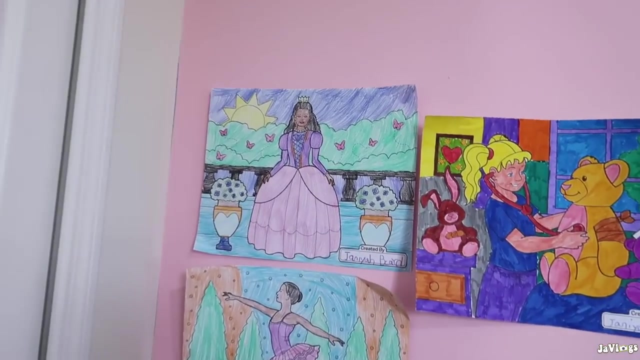 It originally was going to go outside, But look what happened to it. It got damaged by the rain outside. So, yeah, It just looks like that now, But it's okay, And then I have this little rainbow up there, And then I have some drawings that I have. 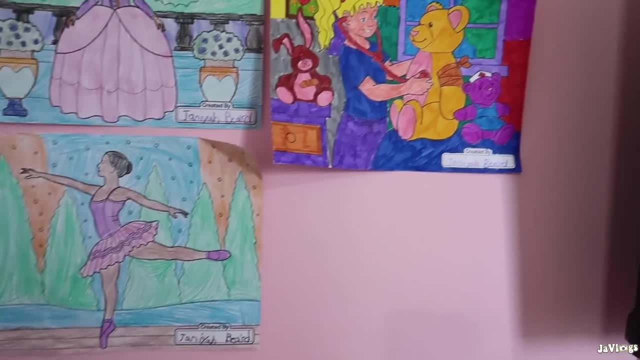 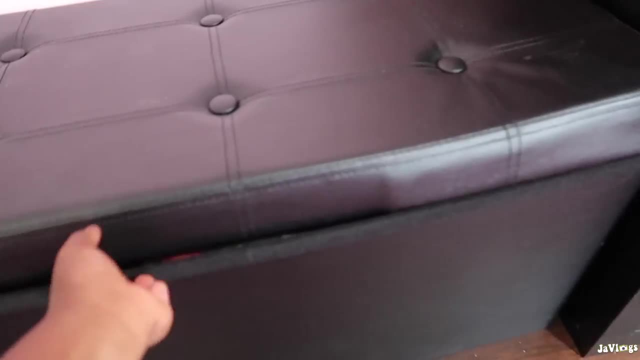 Not drawings, But I colored these from a coloring book. I just wanted to hang them up because they were really cute. I have my skates and my storage bin in here. I just put all of my toys and stuff in there, And then I have my teeth. 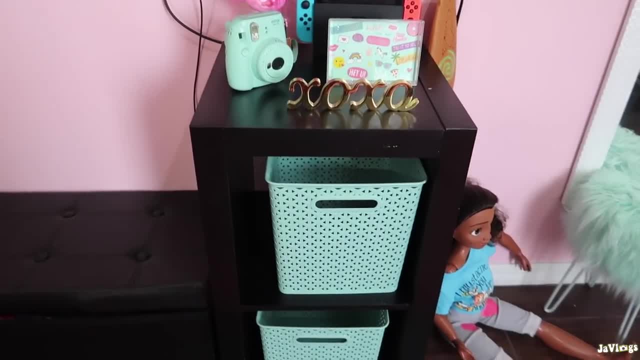 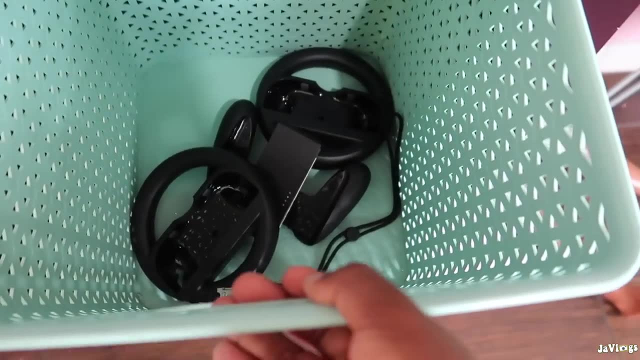 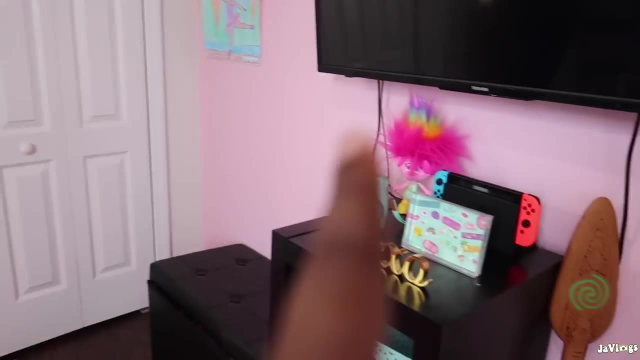 I have my TV right there, Flat skating TV- And then I have my Nintendo Switch- you know some stuff over here- And then I have this bin with my controllers in here and nothing in that basket. So originally this dollhouse was supposed to go over there. 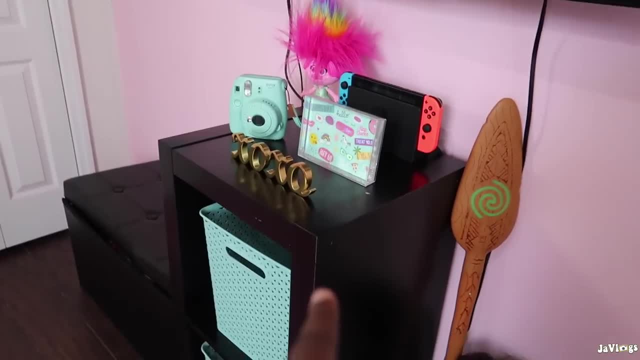 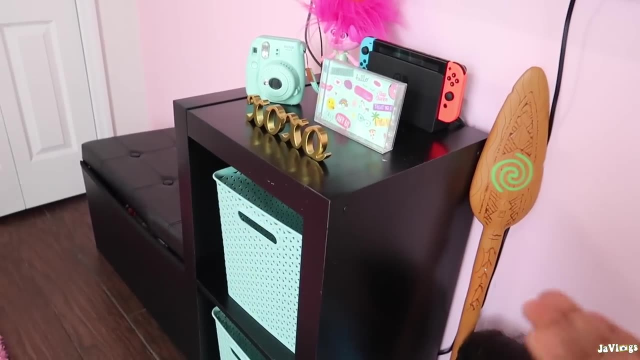 But it didn't fit because of the TV, So we just moved that over there And we put this over here. That was originally next to my bed, And then we have this Moana right here sitting on the floor with her little arm. 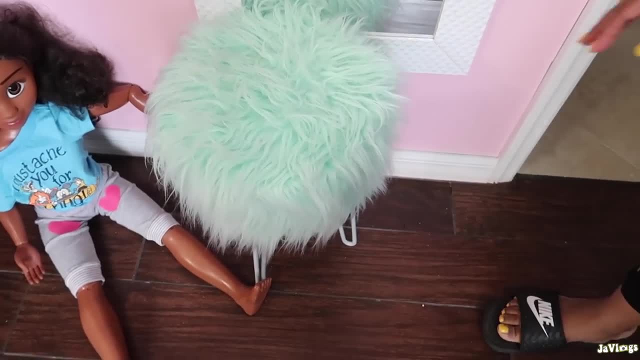 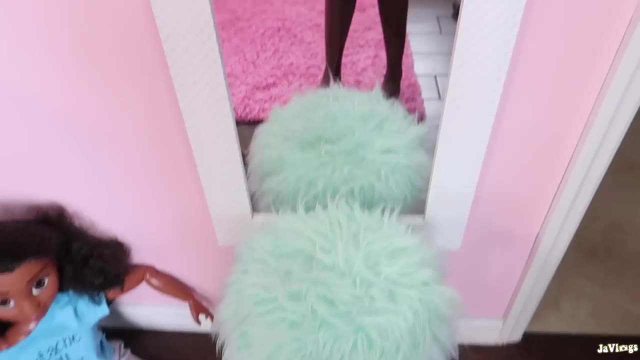 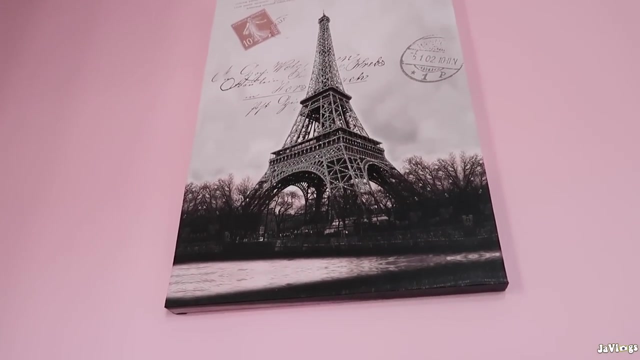 And then this little seat, little fluffer fluff seat, It's a little stool, Yeah, a little stool from Hobby Lobby. And then I have this mirror, And then- oh, I forgot to show that- And then we have this decor with the picture of Paris.